events rather than other ways. This is so important that we are able to learn all about environmental issues. So today I want to talk about- we are all going to know this subject in coming few minutes- and then I will talk about how- how we are going to affect the environment. 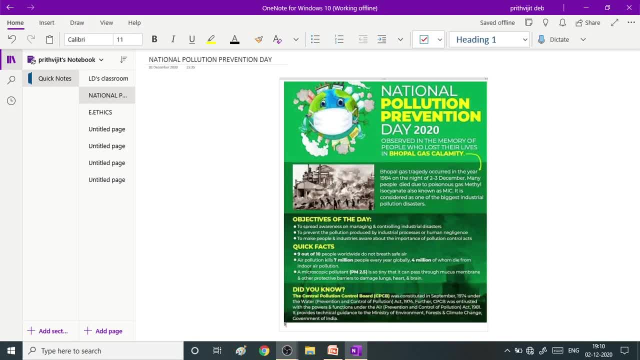 So today I would like to talk about environmental issues and how you can prevent pollution produced by. We are given knowledge about the ways to conserve environment and its resources. Still, we behave so ignorantly that the environment is in continuous path of destruction. So abhi bhi agar hum log ever nahi huye, toh the future generation will suffer due to our activities. 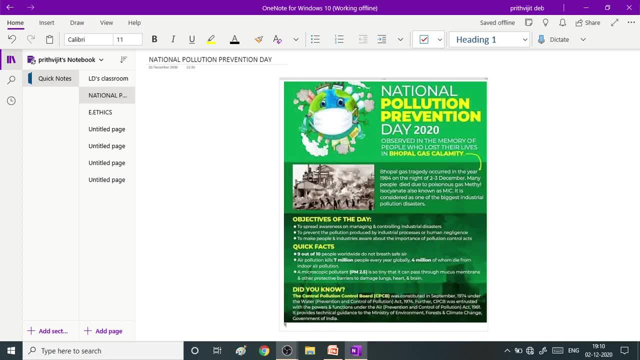 So, no matter in which discipline you are in, you will getting to know about the objectives, principles, aims of environmental education. Aap logon ko formal, informal, non-formal environmental education ke baare mein Patalya, But until and unless we take oath to save environment, hume kuch bhi parhaya jaye. no matter what learning experiences we are taking regarding environment, uska koi matlab nahi rehega. 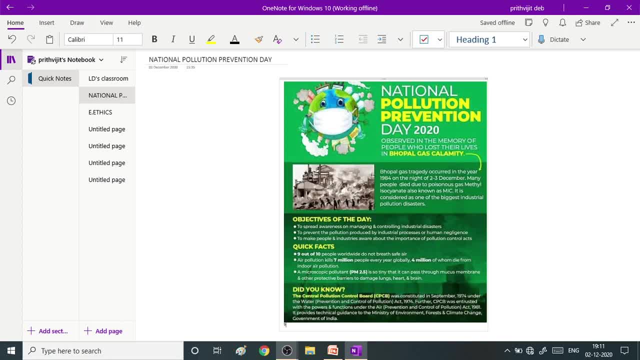 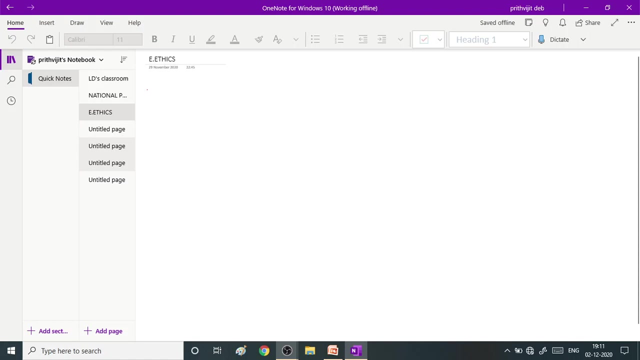 So that is the reason today we will start the video related to environment with environment, Environmental ethics. Okay, I think aap sab ko pata hai ki environmental ethics kya hota hai. What is the meaning of the word ethics? Ethics meaning, the meaning of the word ethics is nothing but some conduct. 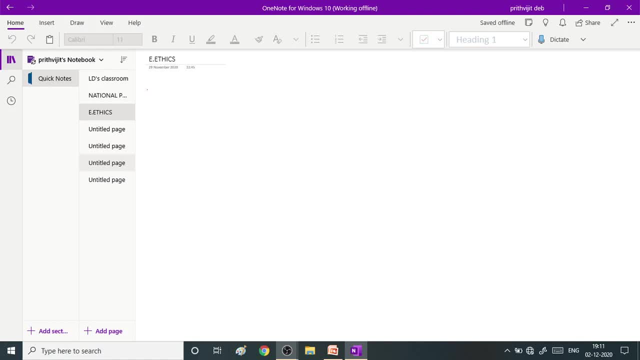 Kuch achar, kuch niti niyam jo hum ko follow karne chahiye, to be ethical with the nature. Or Kyuki, Kyuki, Kyuki. hum log environment ki baat kar rahe hai. So it's not only something like plants, animals or trees or rivers. 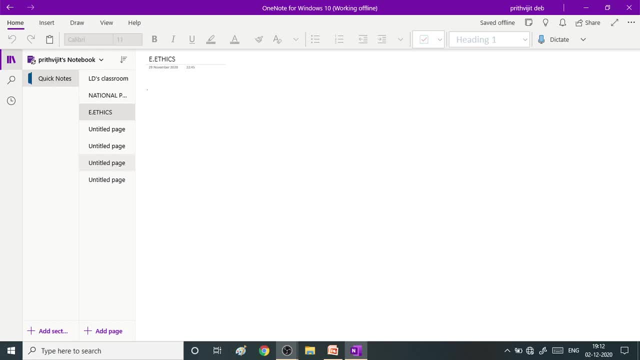 It's something whatever surround us, Kuch bhi humare chaaro, aur hai Un sabhi element ke prati hum logo ko ethical hona bahut, bahut zyada zaruri hai. So Kaise hum, Kya, kya achar vichar hum logo apne aap mein inculcate kare. 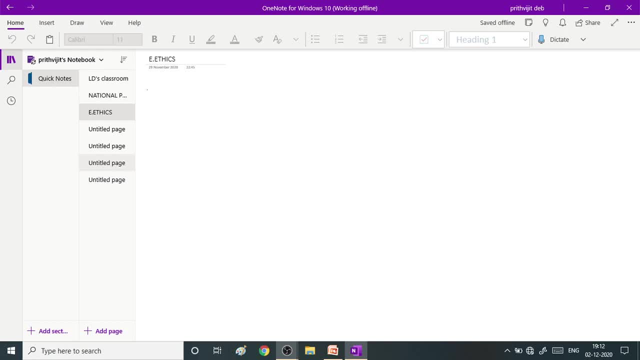 So that we can be ethical to the environment, Because environmentally ethical hona aaj ke din mein bahut, bahut zyada demand hai, Because agar abhi hum log ever nahi huy, Abhi hum log environment ki prati ethical nahi huy. 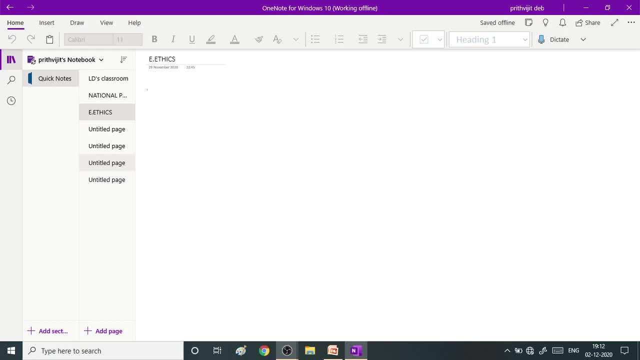 To, it will be Very difficult for us to survive in the world. Okay, So Pehle hum shuru karte hai. kuch principles, Principles of environmental ethics. So many principles are there? A few of the principles I will be discussing. 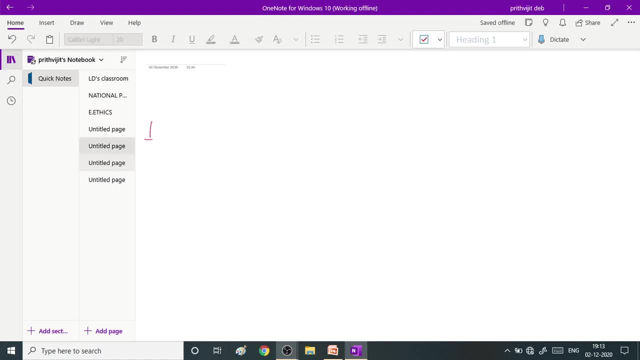 Among those First is Anthropocentrism. Okay, According to this principle, kya hua hai ki human beings ko sabse important element kahe sakte hai Component, kahe sakte hai? Mana gaya hai, Human beings are the most important beings, or baki jo bhi hai living plants, other animals, insects, birds. some non-living components are also there. 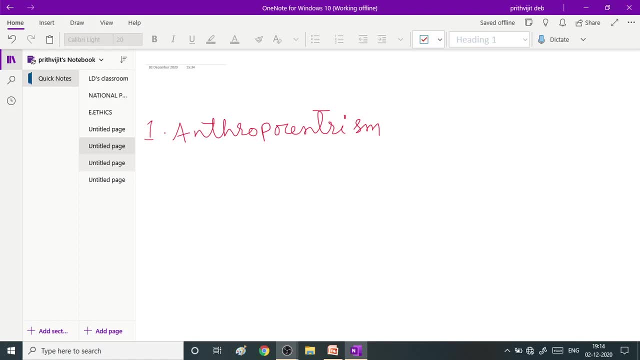 And baki sab ko accessories mana gaya hai, jo ki human beings ko assist kar sakte hai to save environment and also for their survival, Human beings ko sabse upar rakha gaya hai, baki sab assistance hai. Human beings ka kaam hai ki environment ko save karna, so that all the elements of the environment can be saved. 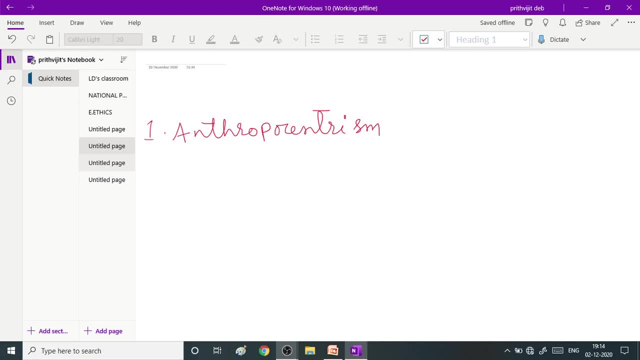 Can be survived or baki jo components hai environment ke unka kaam hai, human beings ko assist karna for their own survival, Again jo anthropocentrism hai. usko bhi do bhaag me. we can divide or we can categorize them into two different parts. 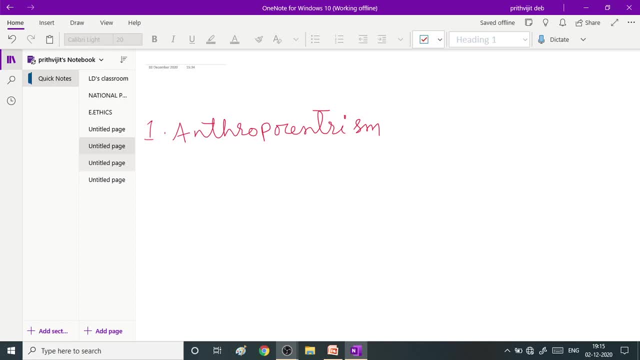 One is strong anthropocentrism And another is weak anthropocentrism. Jo weak anthropocentrism hai wo believe karthe hai ki human beings are the centers, Because unka jo perspective hai. environmental situation ko leke, us perspective ko properly interpret karke, hum kya kar sakte hai? environment ke prati ethical ho sakte hai? 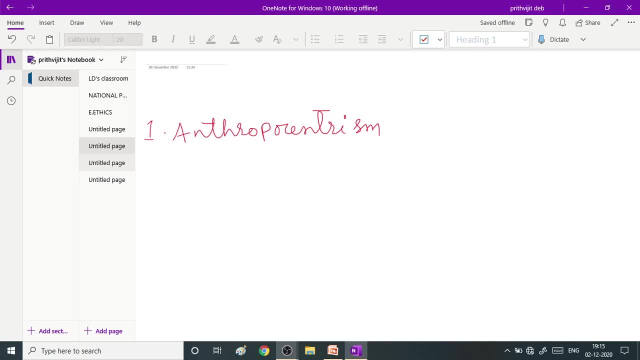 Hum environment ko properly treat karse. That is weak anthropocentrism. Next is strong anthropocentrism. Here the belief is human beings are at the center, because they deserve to be there, Because human beings ko kya mana gaya hai. they are the superior creature. 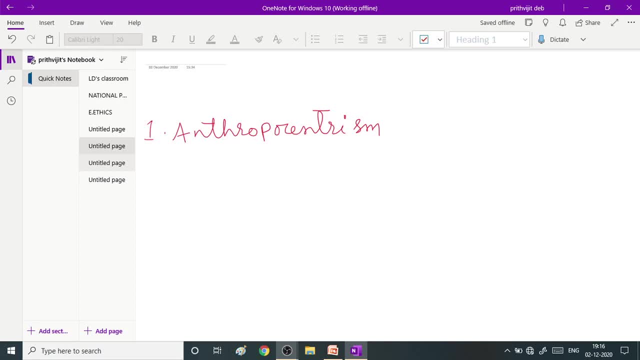 They are the superior creation of God, So human beings must be there in the center of all, All the ethical arena. So this is about strong anthropocentrism. Next, kya hai? Non-anthropocentrism, Non-anthropocentrism. 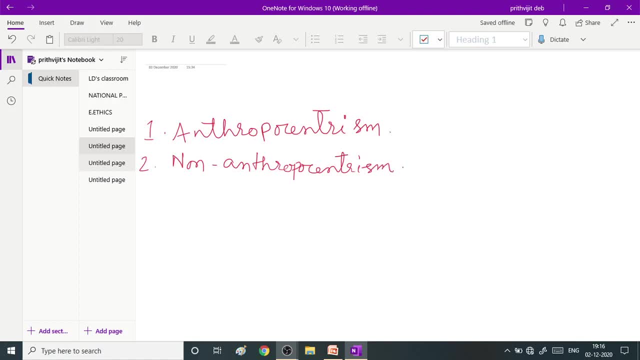 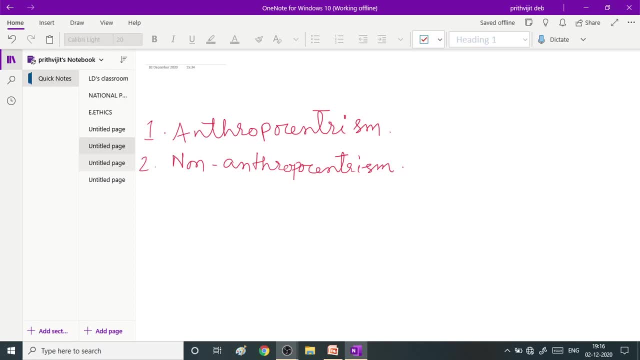 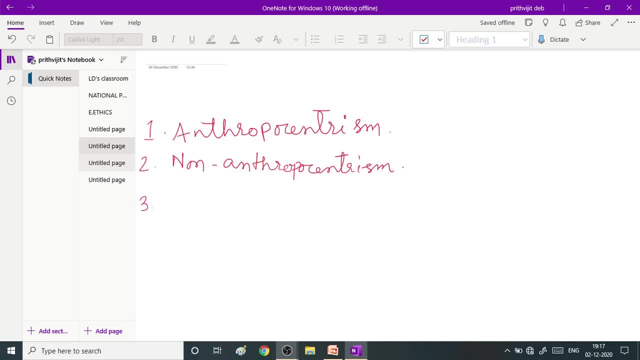 What is the next principle? Psychocentrism. I think you must have known from the name that it is something related to human mind, or you can say mental capacities. So, according to this principle, The human beings. because if you compare human beings with that of the other animals, other animals ke comparison, me human beings ka mental capacities bahut zyada developed, hote hai, or bahut zyada complex hote hai. 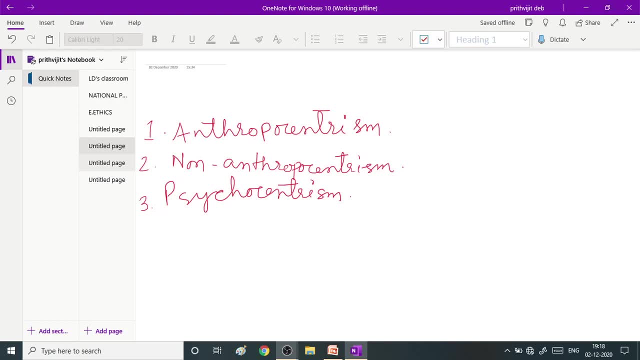 We can think too far. So according to this, that is, according to psychocentrism, The human, that is, human beings, hold more value in the environment, Kyun ki hum logon ka brain bahut zyada developed hai, So hum log bahut zyada, we value more in the environment than that of the other element of the environment. 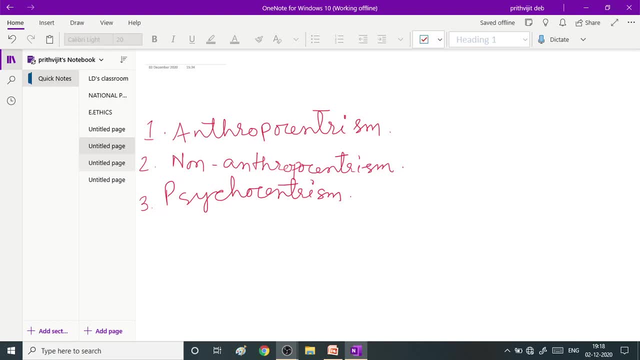 But I don't know whether you agree or not. I strongly believe that we are not doing this, We are not doing the same. Okay, Next, jo principle ke baare me hum log abhi discuss karenge wo hai sorry, wo hai? biocentrism. 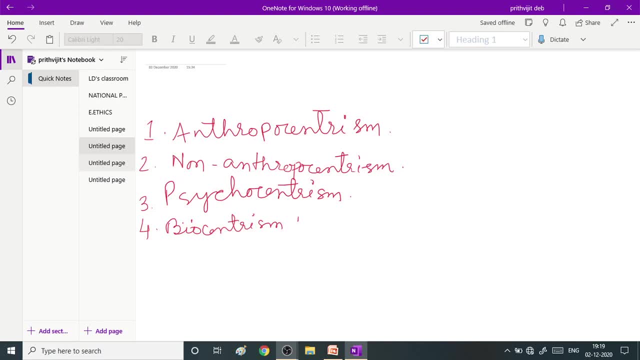 Okay, According to this, I think now also you have understood bio, something related to living beings. Okay, So this is a philosophy that Imparts more emphasis on all the living beings, Though hum logon ko pata hai ki, environment is not something related to only human beings. 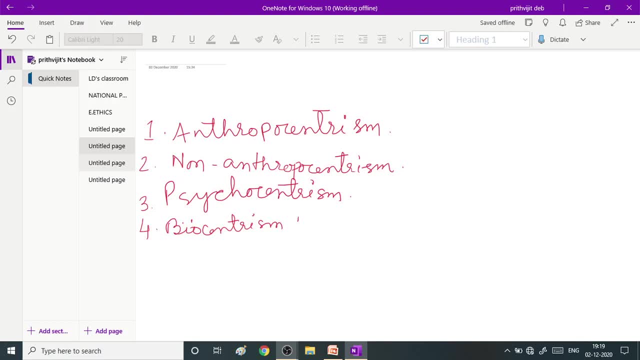 Non-living things are also included in the environment, But still, according to this principle, more emphasis is given to the living beings. So yaha, ye kaha gaya hai ki jo environmental Okay, Pat prati hum logon ko, hum logon ka jo bhi responsibilities hai. 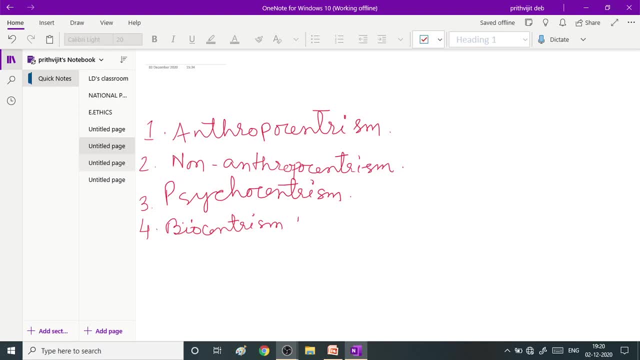 Wo usme political values bhi include karna chahiye. At the same time, we should maintain a proper balance of ecology on the planet. Okay, So this is about the biocentrism. Next, jo principle hai wo hai hollowism? 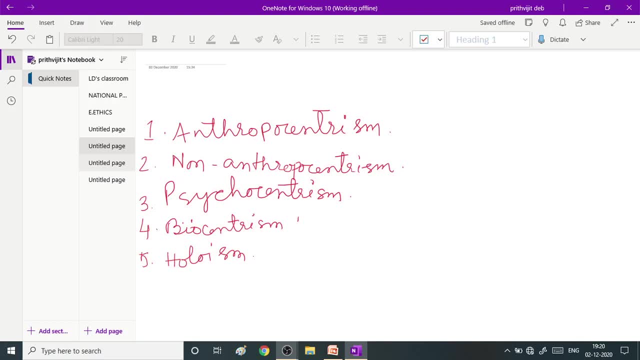 Okay, Hollowism It is. hollowism considers environment system as a whole rather than being individual part of something Jo hum log whenever we discuss about different elements of environment. Hum jab bhi baat karte hai, hum jab bhi environment ke baat baare mein baat karte hai. 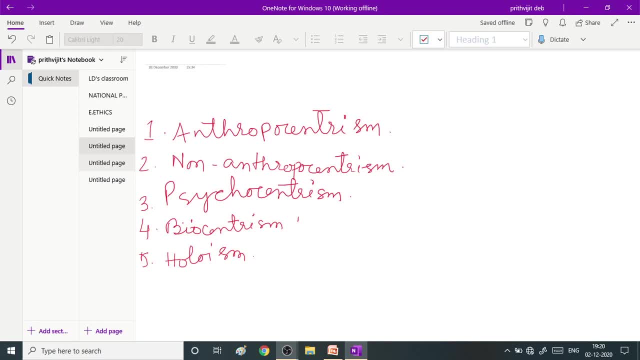 First what we do. we divide the environment into different parts. Hum log bolte hai: Okay, Abiotic environment, biotic environment, phir abiotic environment. ko hum log phir se categorize karte hai: lithosphere, biosphere, then sorry, lithosphere, hydrosphere, atmosphere. 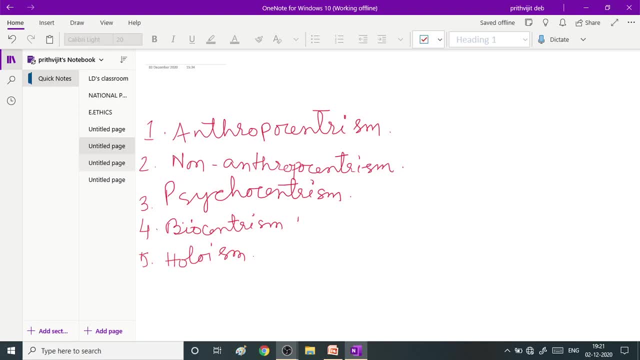 Aise, kya karte hai, hum log environment ko chote, chote part me divide kar lete hai. Lekin jo hollowism hai jase ki hum log education me bhi patte hai ki holistic development, Holistic development. 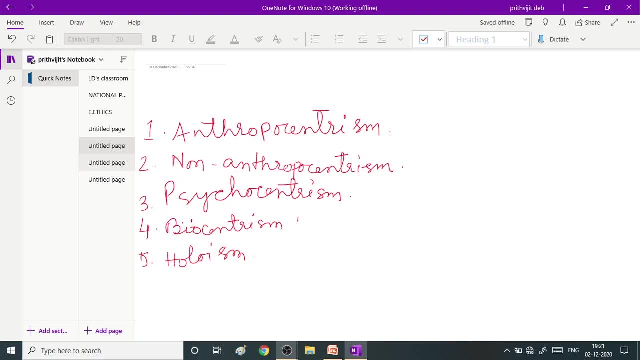 So it's something like that. that is all round Environment here. according to this principle, environment should not be considered as parts. Instead, it should be considered as the whole thing. Okay, So yaha, kya hai ye environment system ko more value add karta hai? ye believe hai hollowism principle ka? 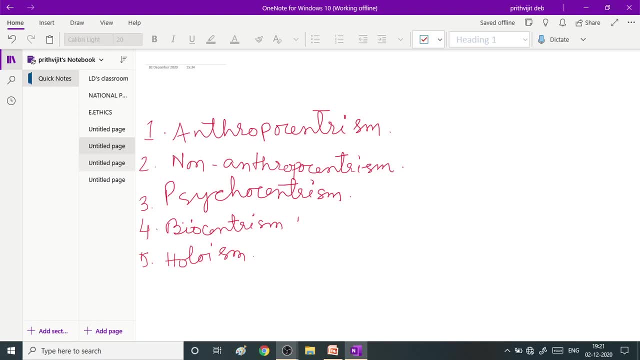 So this is the fifth principle of environmental ethics. Abhi hum jo next hai, that is resource Resourceism. Sorry, Thora Haan. Resourceism, Okay, Resource Resource, Ye jo principle hai. Woh kya karte hai ki nature is considered to be valuable only because it has resources to provide with. 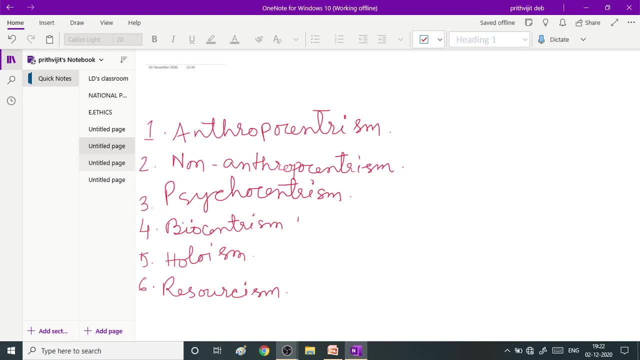 To for our survival, hum logo ko survive karne ki liye, whatever necessary requirements we have, All the things we are getting from environment, Hum logo ko environment resource provide karta hai. Isi liye hum log Ko ko. 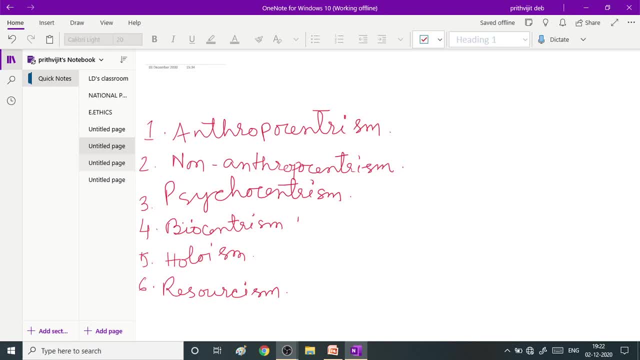 Environment ke prati ethical hona chahiye. Aur resourceism, ye bhi bolta hai ki nature. thus what is happening? because we are getting resources. that is why we are exploiting the nature. Okay, So, instead of believing in taking only, 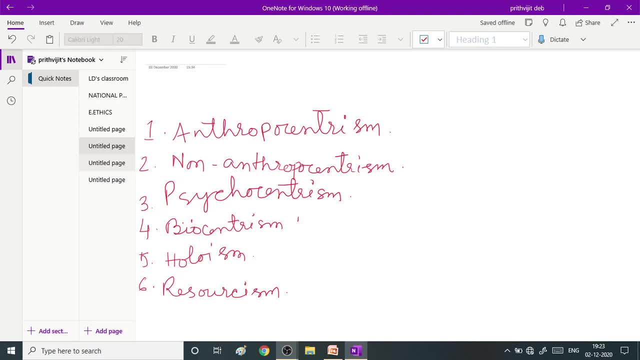 What ye? kya ho raha hai ki hum log abhi jo relationship hona chahiye, Hum humare aur environment, or between us and the nature. it should be give and take relationship. we should take something from the environment or nature and in return we should give something also, so that ek balance rahe. 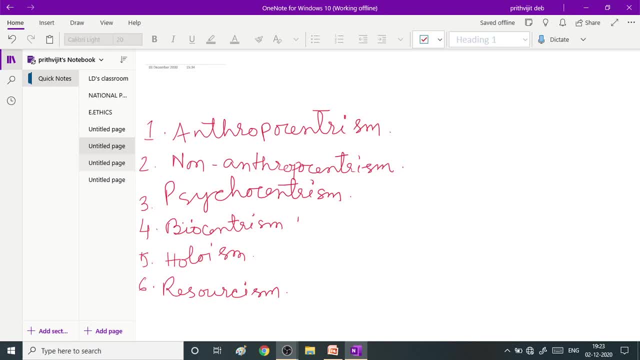 So abhi kya ho raha hai? kiuki hum log har resource, hum log nature ko value isi liye karte hai, kiuki ye humko resource provide karne. So nature is ought to be exploited, Okay. 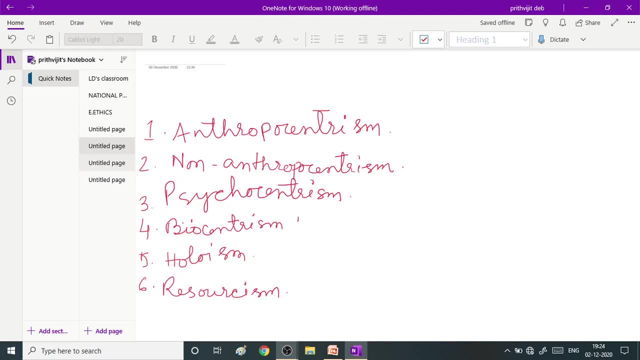 So that should, that is, according to the principle of resourceism. Jo next principle hai speciesism. Okay, This word, I think all of you know about the word species. Okay, Okay, This particular principle, ye kya hota hai ki human superiority, human race, jo hai unki superiority ko, superiority ko justify karta hai. 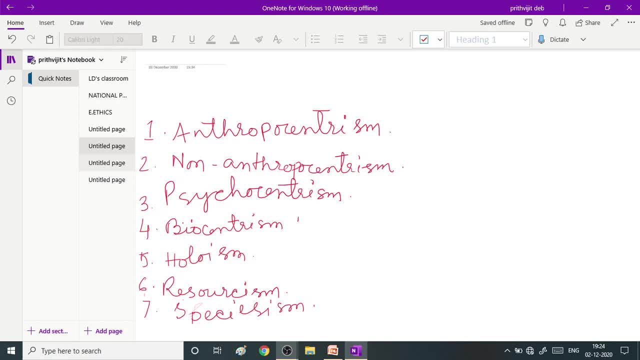 It also justifies exploitation malnutrient of animals by mankind. Kiuki hum log bahut superior hai. we can do anything. We can exploit the nature, We can exploit the other Animals or plants or whatever other living creatures hai ye principle ye justify karne ke koshish karta hai, which is very negative. 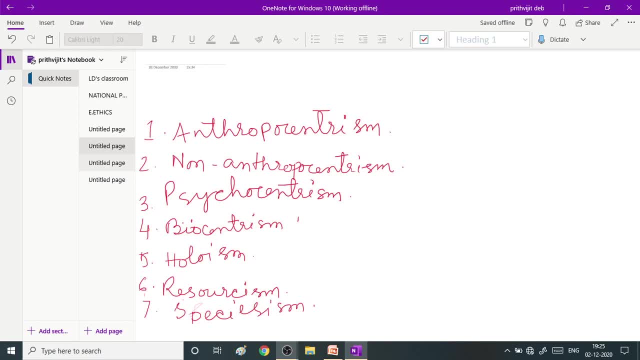 They say that because we are the superior creature, isi liye hum log kuch bhi kar sakte hai. But this is not the thing. actually We, because we are the superior creation of the God, It is our duty to be responsible to the other creations. 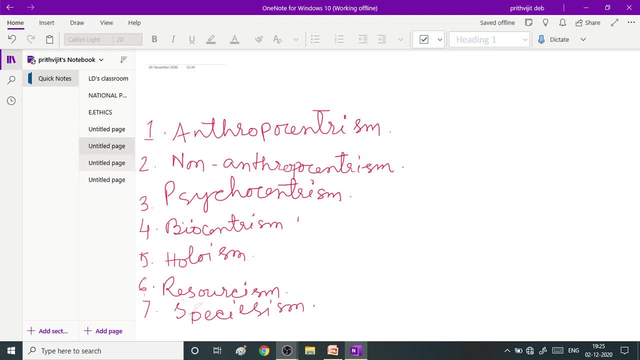 If hum log agar other creations ko inferior maante hai to being superior, we have the responsibility to take proper care of the other inferior creatures of God. But speciesism ye nahi maante hai, Because if we are the superior of humans, do not take our third�I reach to freedom. 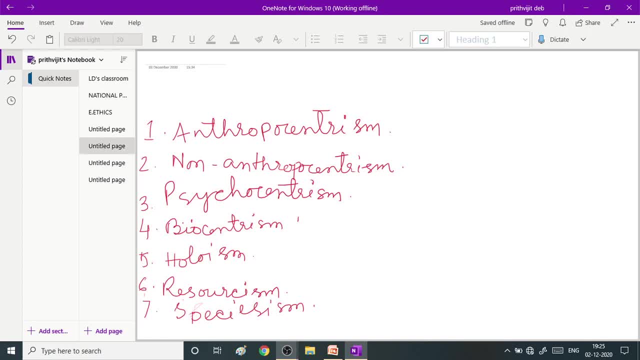 Even elders and village clever just like us, Astron and Kyle and so on… ідने पण यी पतनवालु भOOK. हर भूइर आचू कर दिस त्यू. 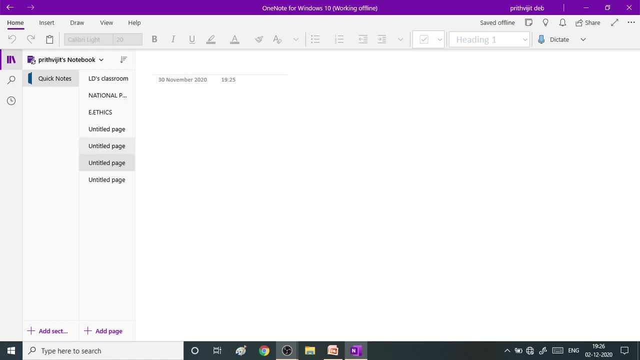 Memesis is event evaluation, utilization, development, 얍छा procrastination for developing and Czyli fantasy system. पपा 쓸ाद वग्या बर्गा इकप्राण करूंगे परा कर दि CORRECT CONSIDER IT. 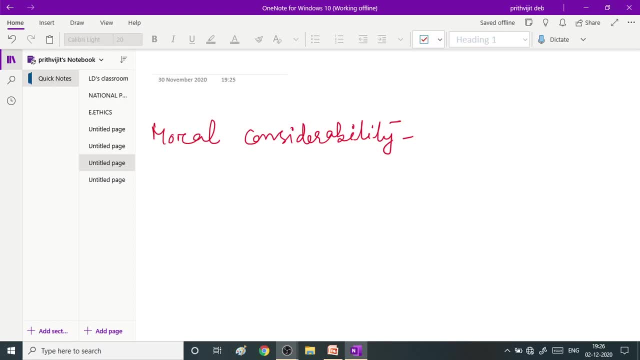 principle is environmental ethics, the intrinsic value that we should feel for the other creatures of the environment, Like what happened in the Chipko movement. they were feeling from inside that the plants are something of our own. So the intrinsic value that comes from inside when we feel other creatures also as our very. 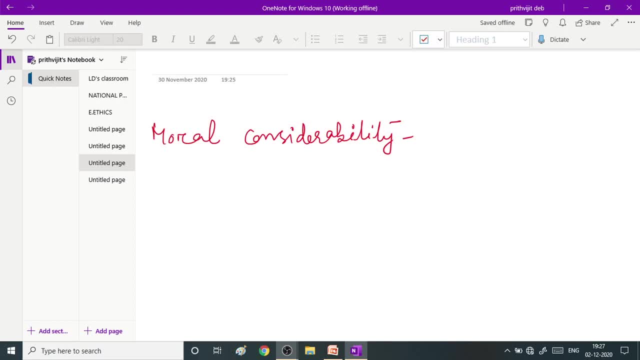 own. So this moral considerability, what does it agree? that we, no matter whether we are superior or not, but all have equal rights on the natural environment And our feelings for other creatures are moral considerability, injuring the sexes, the sexes that come from inside? 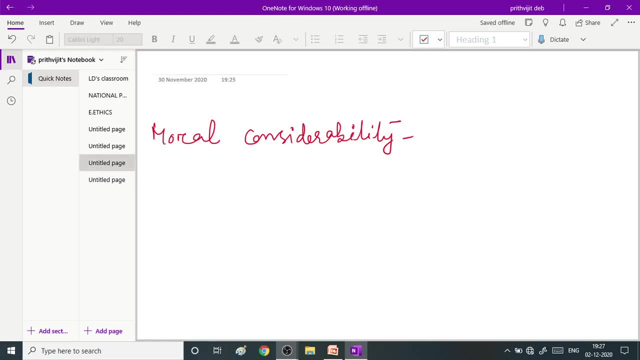 So this is moral considerability. Next is actual balance, and that is the most important thing. That was number eight, This is again number nine. This is instrumental value, this is moral value And this is the next and most important one. 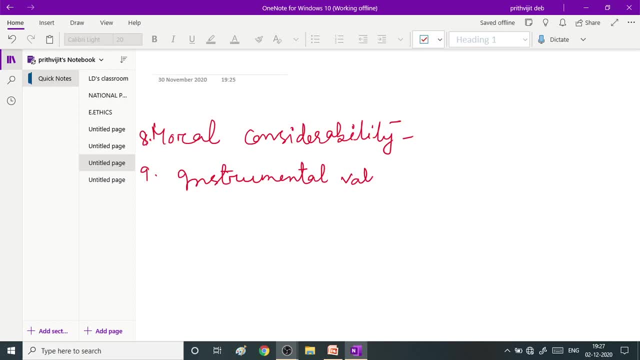 This is about moral value, And here the next thing that I will be discussing is the moral value. Okay, Instrumental value is something that is imparted? Okay, That is imparted to a being as long as it can serve us with resources- Okay, Whatever resources are there. 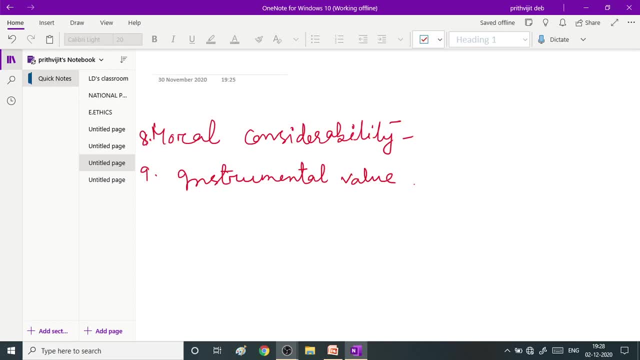 How long can we provide these resources? How can we conserve them so that it can be all the resources can be preserved for the future generation also? That is mainly the concern of this principle of Environmental ethics. Next is intrinsic value. Okay, It's just attached to a being. 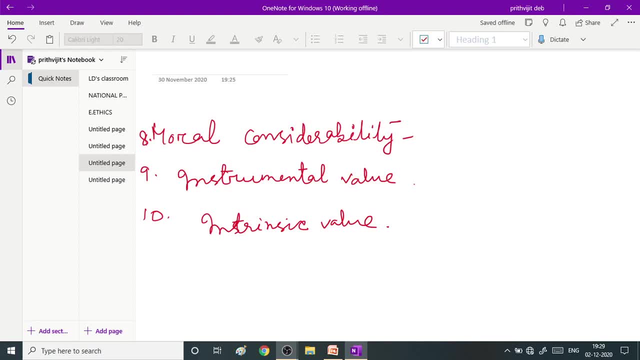 The available in the nature, The characteristics like resourcefulness of nature is not just for us but also for other creatures. Okay, So these are some principles of environmental ethics. Now I will tell you- It will be a little simple discussion- That we have become very bookish. 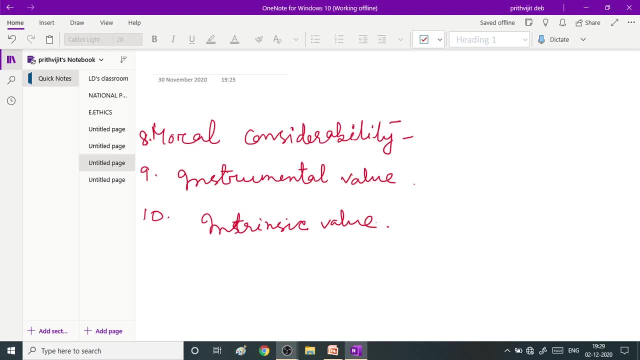 Still, you should know About the principles. Now we will discuss How. What are the behavior We should inculcate in Ourself so that We can be Ethical to the Environment? Okay, So the First point. 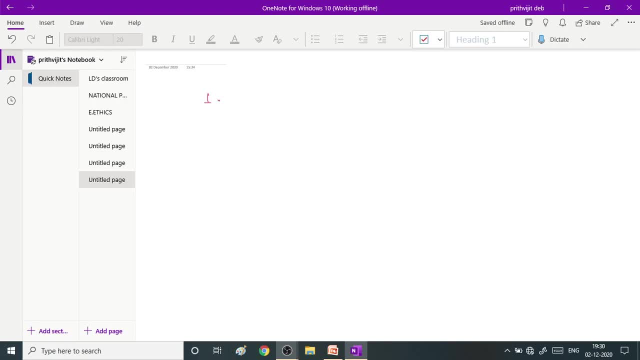 That comes in our, That should come in our Mind that We should love and Honor the Earth. We should love and Honor The Earth. So Now you ask yourself. We always say Mother earth, mother nature. Whenever we, With the earth And with nature, We behave the way We do with our mother. No, never. There are a few Peoples- you can Cite examples of a few People- who behave The earth or the Nature as their. Mother. Okay, So We should do, Because See why we are, Why We are indebted to our Mothers. We Mother Because Whatever requirements We have For our survival, That all the necessary Things we get from our mother. 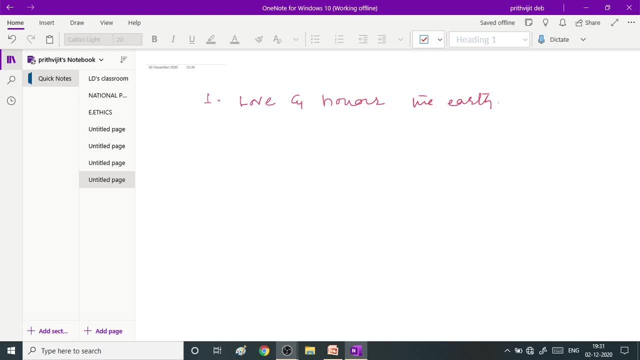 So same thing earth Is also doing for us. So what is the problem? To feel the same way, for the earth, To feel the same way, To be responsible For our mother. So first We should Love the mother And love the earth. Since Earth has blessed us With life And governs our survival. Our Life and survival- All These two things Are blessings of The mother earth. That's why We must love And honor the earth. We should not. 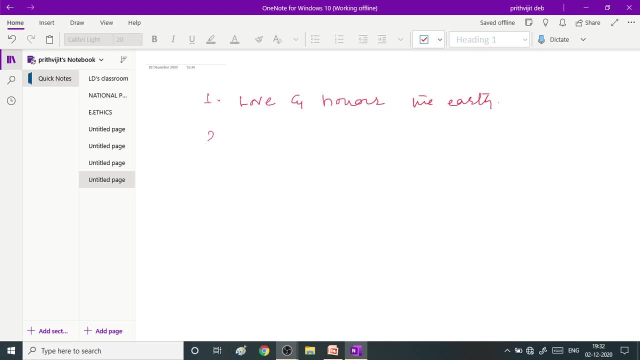 Love And honor the earth. Because We are getting something, Take care of it. Don't do it Selflessly By keeping in mind That something we are getting. That's why we should- In return, We should- give some. 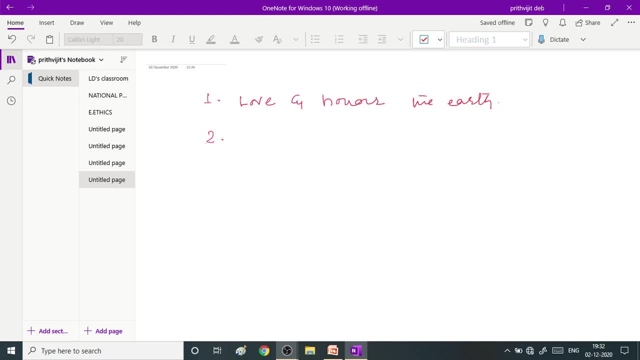 Love and honor to the earth. Next is: Celebrate to earth And should Celebrate the turning Of its season. Okay, So that is very, very important. We Celebrate a lot in the year, Like Holi. 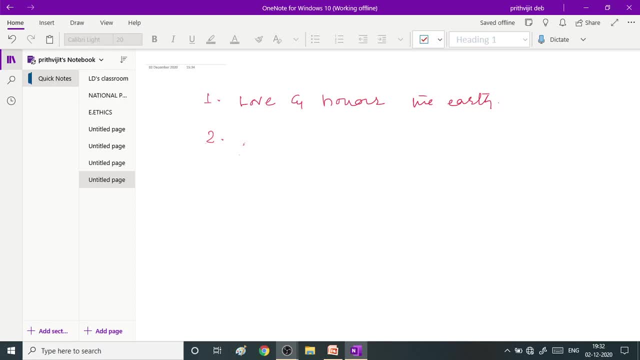 Like New year, Our In Assam, Like In South India Pongal. There are many such Celebrations. We celebrate that. But why we do that? We are not aware Of those things. Holi is celebrated to welcome. 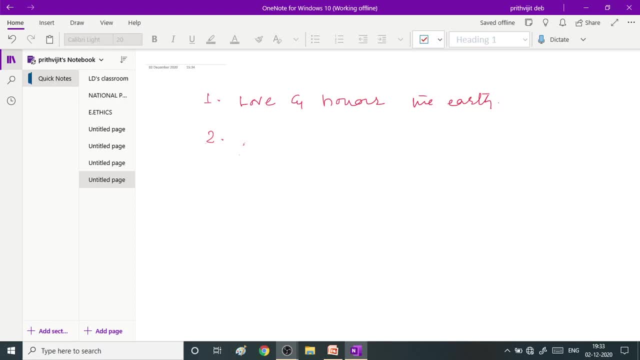 The season of spring, We welcome the color Of the nature. What happens in spring season- All four, So many things- Gives color to the Surrounding And that is the reason Holi is celebrated. It's not like. 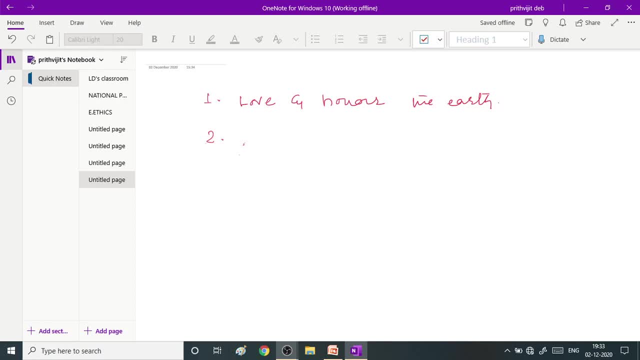 We played Holi, We did some function, We did some party, And that's it No Why we are doing all these things. We should have some secret feelings In our self While celebrating. Okay, You have heard Social festivals. 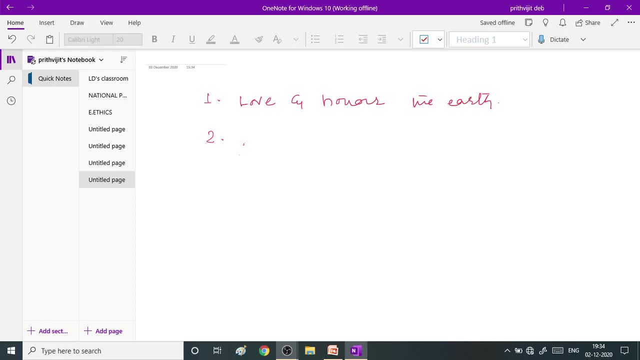 Many regional festivals. This is Natural festival, Which we should Celebrate with Many sacred feelings. That brings our self More close to the nature. Okay, Next, We should not hold ourselves Above other living things And have no right to drive. 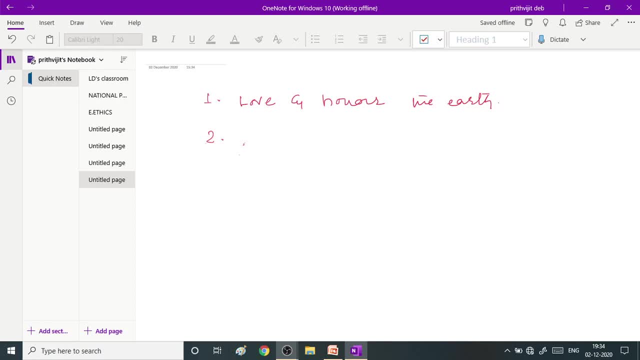 To drive others To extinction What we are doing now. So many animals and plants, Some have extinct From the world, Some are endangered, Some are vulnerable. Why such things are happening. All these things are happening Due to our activity. 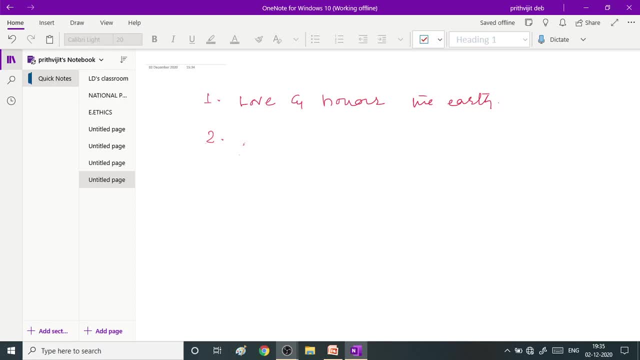 Do we really think That we are superior And on earth, What is that We should rule? So We, without any hesitation, We forget That it's not We like other. We are not something very superior Like us. 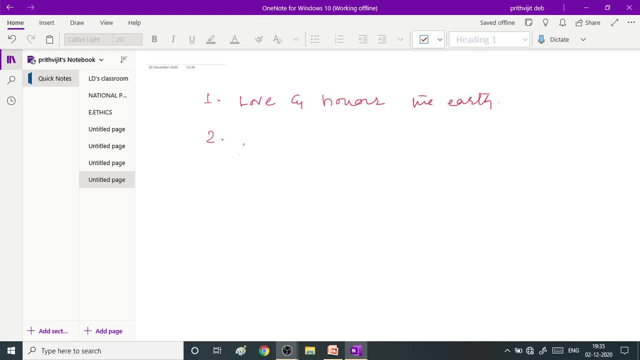 Other creatures also have the same right. Like for mother, All children are equal, Similarly For mother nature The status of a human being, That is The status of a small insect. So We should not forget that. So what we are doing, 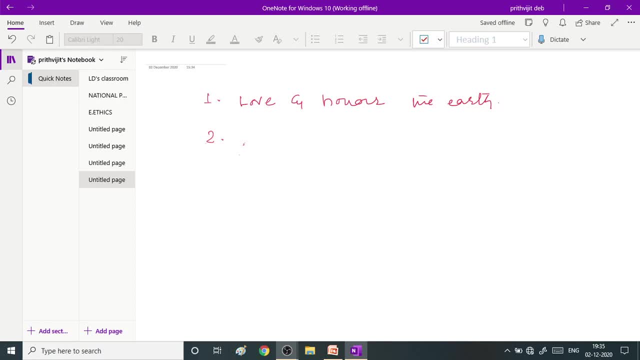 We are becoming very unethical. By Keeping ourselves At the superior position And Without any hesitation, We are Stealing the rights Of other Creatures of the earth And leading them To the And driving them to extinction. 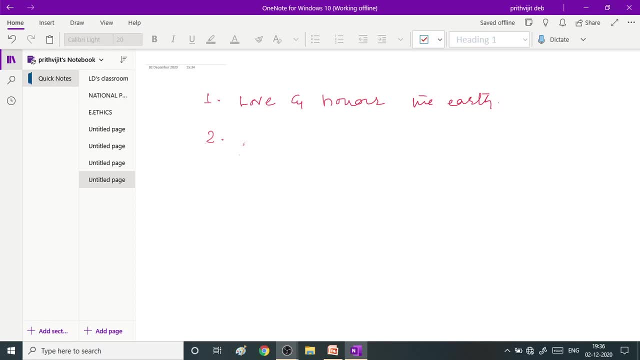 Okay, So that should not be done. See, here, I am not writing the Points. I am not being able to write the points, But While listening to the video, While listening to it, You can Repeat it. I am on the whole sentence. 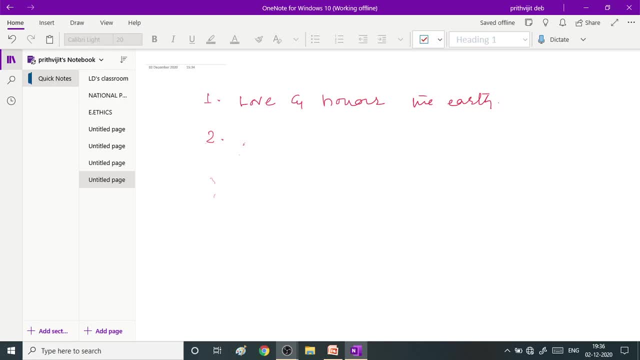 Okay, So the last point: We should not hold ourselves Above other living things And have no right To drive them to extinction. Next, We should always Be very, very grateful To the plants And animals. Who nourishes us by giving food? 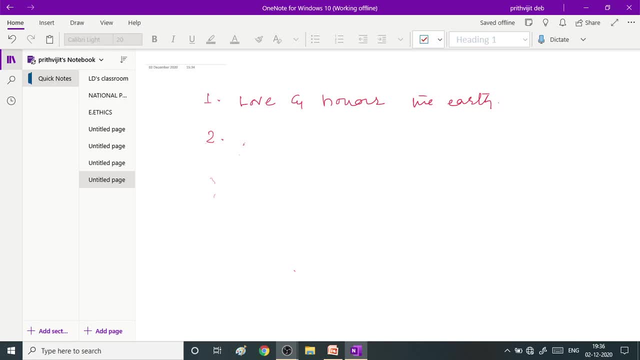 See, we are Directly, indirectly Depending on the plants For our food. At the same time, We are depending on other animals Because we are superior, We have to do a lot of work, So we need more food. So 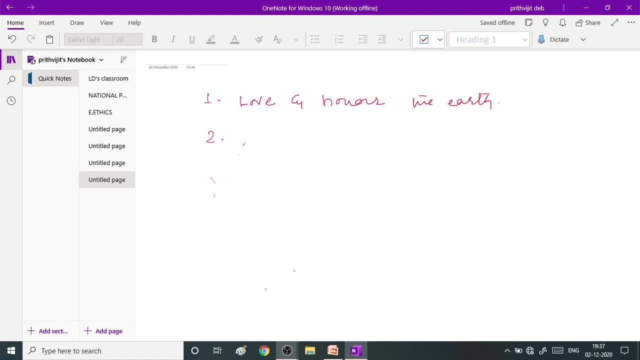 We are completely depending on These other creatures, No matter whether it is a plant Or animal, So we should always feel Grateful for them. We never show gratefulness When we eat a lot of mangoes On the next day. 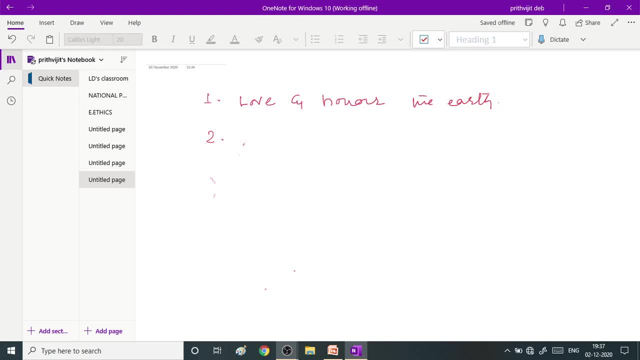 We don't have any hesitation To cut it. So that should not be the thing. We should be very, very grateful. We should be grateful That, to keep us alive, Whatever food We are getting, We are getting it from these people. 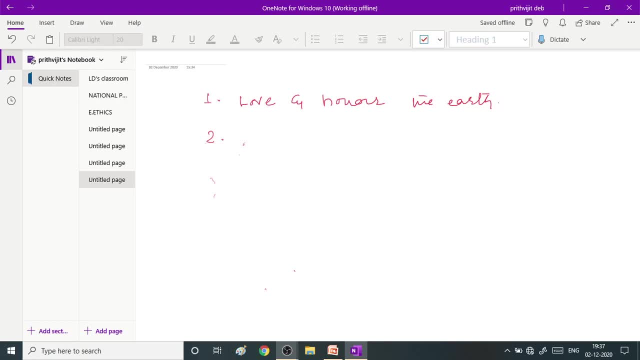 Because of these people. So that is a very Important thing: To be ethical Towards the environment. Then We should limit our offspring, Because too many People will overburden The earth. That is a very, very important thing. 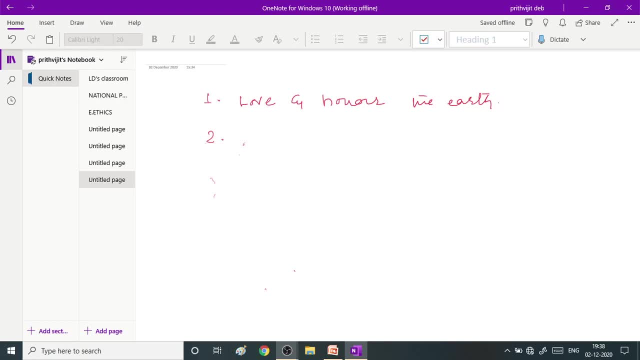 That means our population Should be limited. Whatever environmental Problems are happening, No matter Whether it is something related to pollution Or, You can say, Scarcity of resources. Whatever is happening, That is happening The population of human beings. 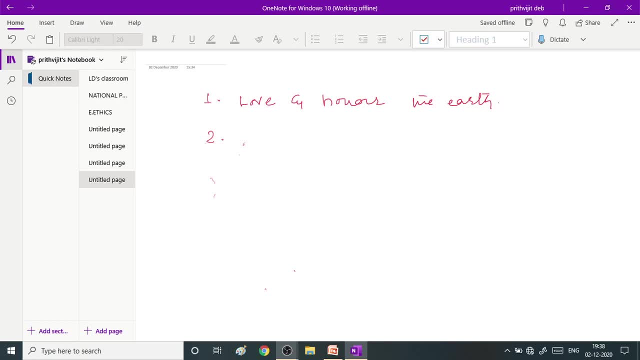 Is very much Unlimited population. Because of this, All these problems are being created. So what should we do? We should limit our offspring So that We don't create too much burden On the earth. The earth As much as it can take. As much as it can take. More than that, Then It will be An unethical act On environment, Or you can say nature. Then we should not waste Our resources On making Destructive weapons. These days It is happening too much. To The Worldwide, To show the Superiority, To show power. Which country has How much destructive weapons? That country, Who has more destructive weapons? That country Consider themselves more superior, More powerful. But that is not an ethical act. 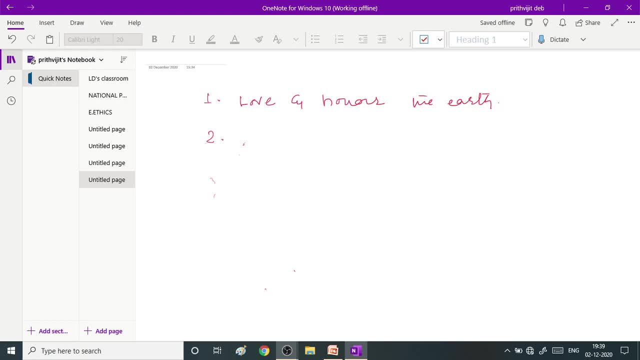 Environmental Ethical act Is conserved As much as The earth, That is, Natural resources, As much as flourishes, As much as enriches, That country should be given Superior place. But It's a matter of 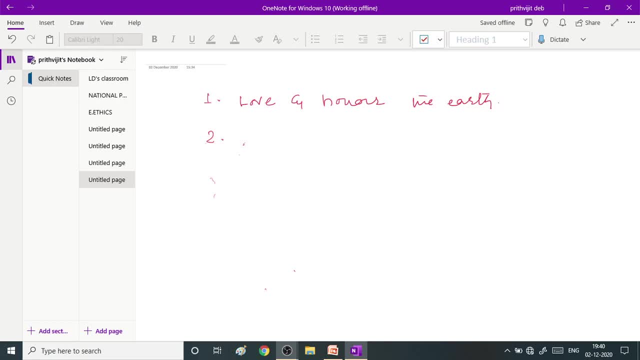 What to say. It's a very sad thing That in practical sense, This is not happening At the cost of Nature, Rather To restore Its damaged Majesty. That is very important. This is going on too much Because the 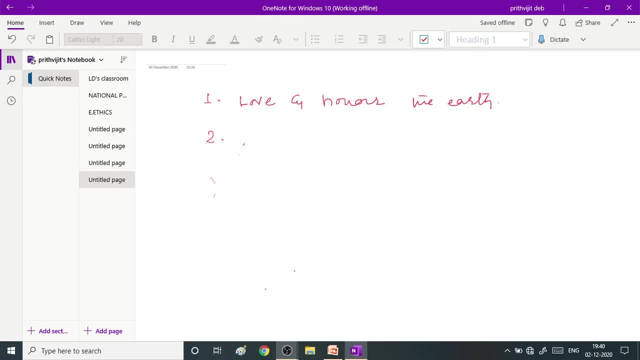 Poaching, Hunting. Ultimately, What is happening At the cost of nature? Gaining of money simply to earn money? What they are doing, They are destructing the environment. Sometimes we are facing many such incidents nowadays. The forest rangers, those who are 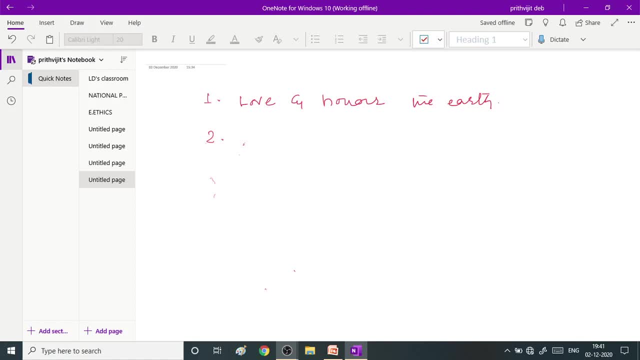 given the responsibility to restore or to conserve the forest resources. what are they doing? They are selling natural resources- animals- for a small amount of money. So that should be stopped. That is an unethical behavior towards environment. Now we should. next. 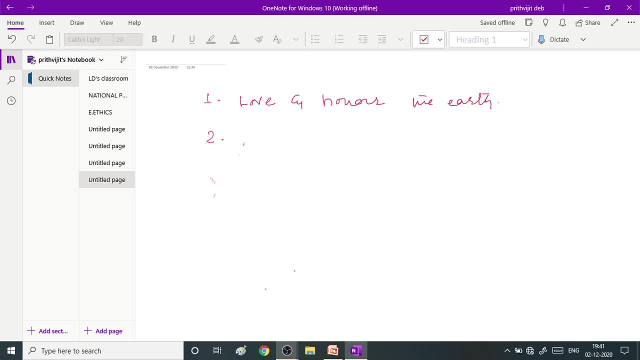 point is we should conceal from others the effect we have caused by our action on the earth. Okay, So that is again. we should conceal from others the effect we have caused by our action on the earth. Okay, So that is again. we should conceal from others the. 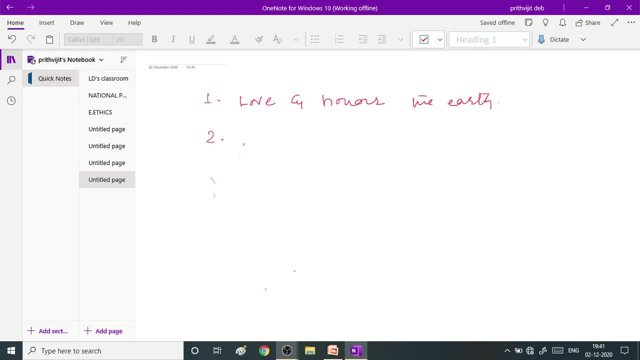 effect we have caused by our action on the earth. Okay, So that is again, we should conceal from others the effect we have caused by our action on the earth. Okay, So that We need to be regretting, we need to feel ourselves bad, that hum logon ke liye un logon ko problem ho raha hai. 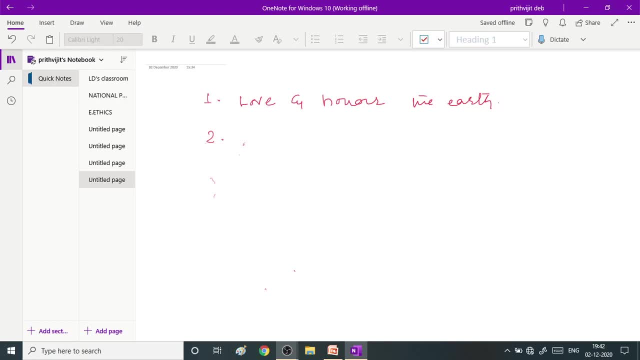 Then we shouldn't steal from the future generation their rights to live in a clean and safe planet by improvising or polluting it. So what is happening Aaj kal? ke jo parents hai, un logon ka kya hai ki bachay ke liye bahut zyada properties, bahut paise, bank balance, rakke jaa raha hai. bachay ko koi problem nahi hoga. 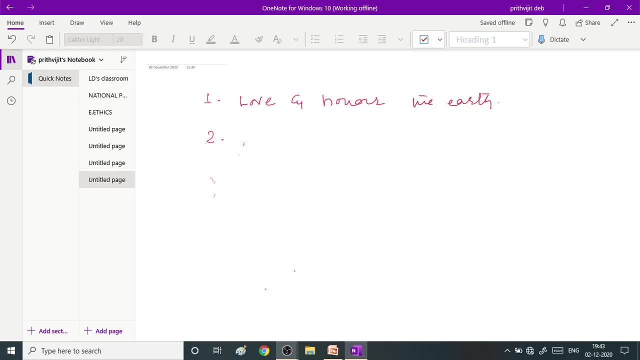 In logon ko yeh samaj mein nahi aata hai ki aaj se, 20 saal baad, jab tumhare bachay ko khane ke liye paani nahi milega, saas lene ke liye fresh air nahi milega, to wo yeh paise aur properties se kya karenge? 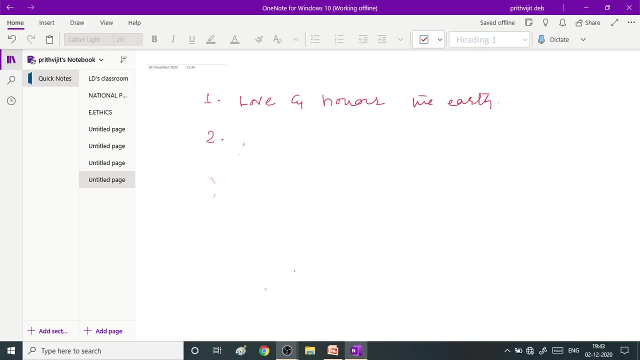 So every parents or the members of the current generation must think like this: Kyuki ek ad aata tha kuch saalo, pehle bachay apne papa se kera hai ki mai jab bara hunga mai cycle ki dukaan khulunga. 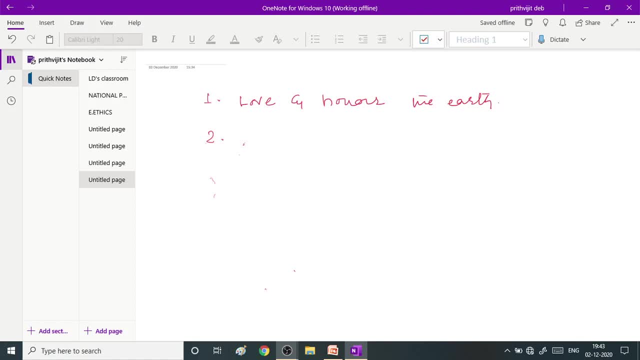 Lekin unke jo papa, the pehle, jab wo unke papa se baat kar rahe hunga, shayad wo keh rahe hunga, ki mere barhe hokar gari hoga. 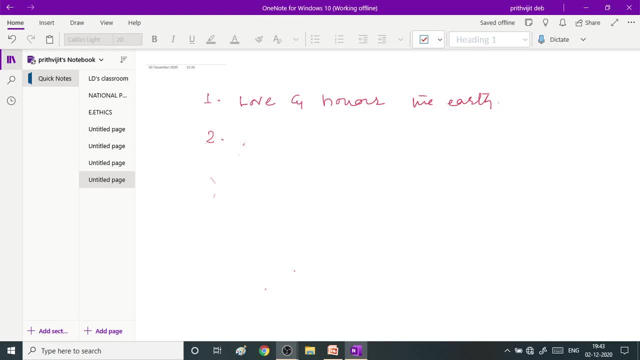 mai gari kharidunga, Lekin yaha dekhiye ki unka bachay bol raha hai ki barhe hokar cycle kharidenge, Kyuki gari chalane ke liye to petrol hungi hi nahi. 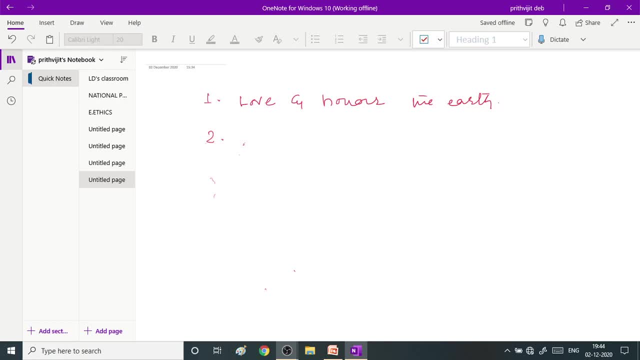 to petrol kisne kharj kia. So that these are the things we should keep in our mind and need to be very, very ethical. Hum logon ko. jo bhi natural resources hai, We should conserve them and should preserve them for future generation. 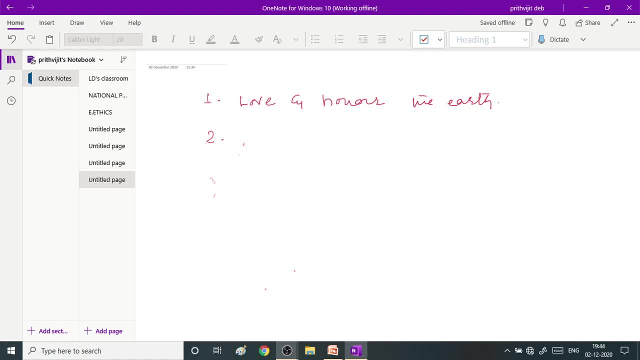 Kyuki jo humne. whatever facilities, whatever comfortabilities we enjoyed by using the natural resources, that comfortability our future generation must also get Okay. Next and the last point is we should consume the material goods to moderate amounts, so that all may share the earth's precious treasure of resources. 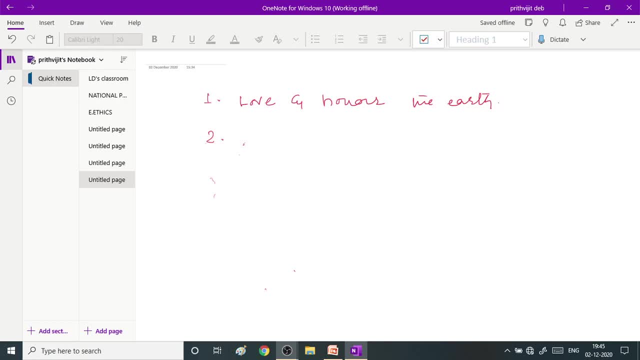 So abhi kya ho raha hai? jo ELITE class ke log hai, Unn logon ke paas bahut zyada paisa hai. Yeh log kya karte hai? Zaroorat se zyada cheeze kharid lete hai. 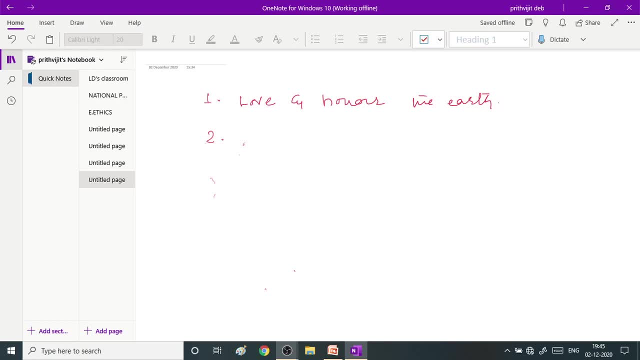 So what is happening? The resources become scarce. So when the resources become scarce, it becomes Very. that is demand full. Iska demand bar jata hai. Jab demand bar jata hai, to cost bhi bahut bar jata hai. 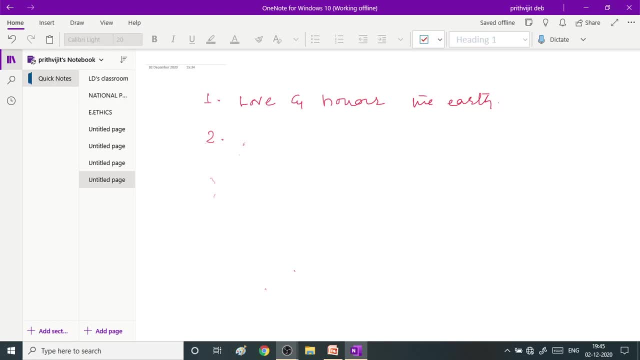 So jinke paas, wo expense BR karne ke liye paise nahi hota hai, Wo ultimately kya hota hai? They cannot get, they cannot consume or they cannot get facilitated from that particular resource. Okay, So no matter how much money I have, 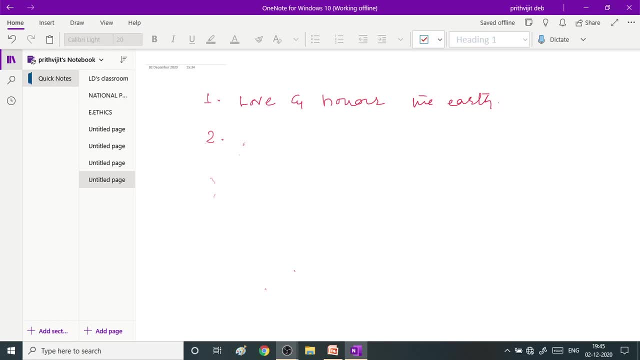 Aaj main mahine mein paas 5000 rupee electricity bill de sakte hoon. To iska matlab, yeh nahi ki main 5000 rupee ka hi electricity bill kharj karu. Kyuki, yeh jo electricity hai. yeh, that is not my own property. 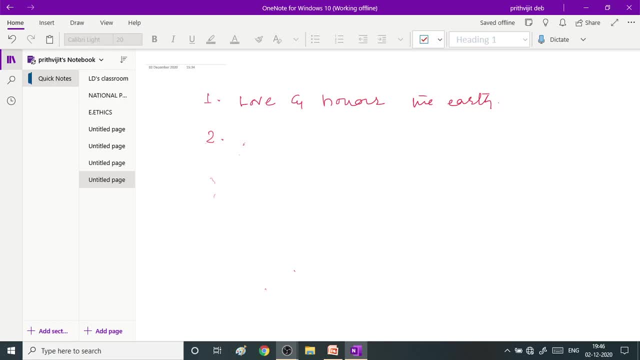 This is not my personal property. All the human beings have equal right. Okay, So we should be very, very aaj mere paas, 10 gari hai chalo, 10 gari leke bahar chalte hai Ek member ke ek family ke 5, kuch saal pehle Guwahati me because I belong to Guwahati. 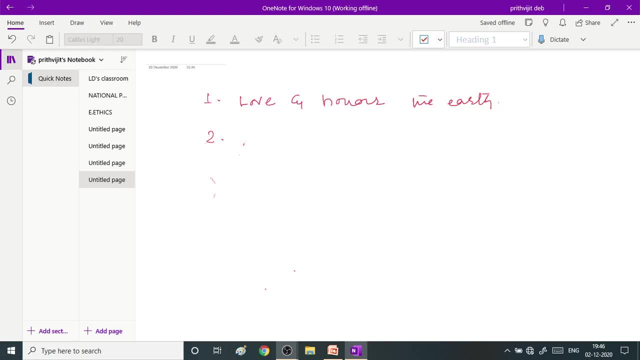 I am the resident of Guwahati. That's why kuch saal pehle ek news channel me ek data transport transportation department May be, I am not very sure which department circulated that data. Waha us data ki hesaab se jo Guwahati hai usme har par head ek kar ke card hai. 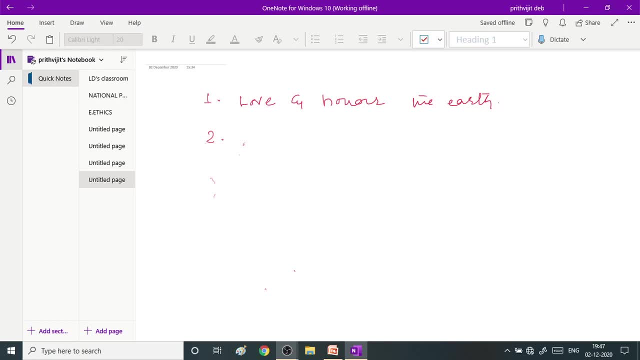 Kisi, kisi aise bhi families hai, jaha, 5 log hai, 5 members hai and there are 5 cars. So, because they can afford, That's why they are purchasing. But this 5 cars, what is happening? They are polluting 5 times.